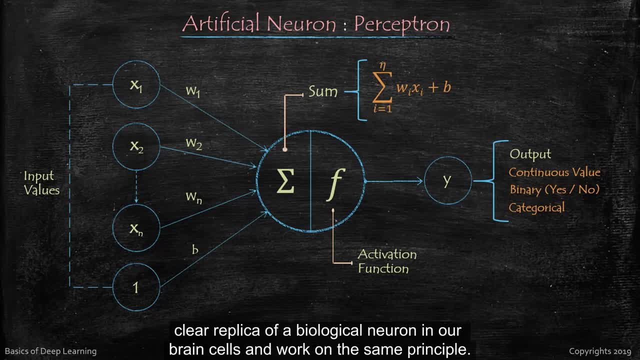 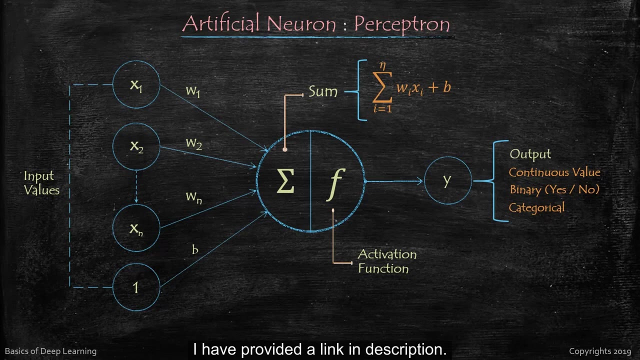 replica of a biological neuron in our brain cells and work on the same principle. To get more details, you may need to watch my previous video on biological neuron versus artificial perceptron. I have provided a link in description. So, as said earlier, a perceptron, also known as a linear binary classifier. 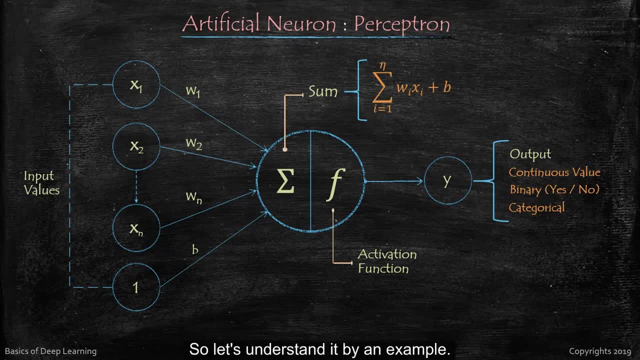 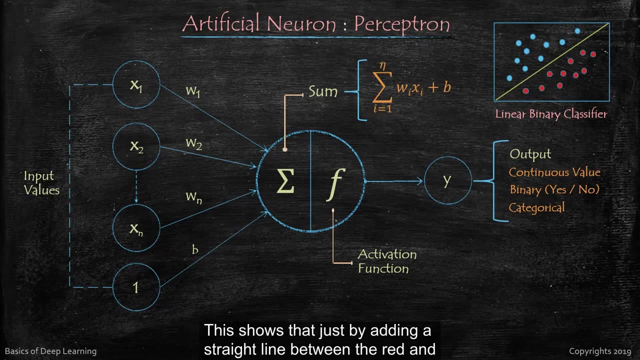 You may ask: what does that mean? So let's understand it by an example. We have a data set, as shown here, with few red and blue data points. We use a line to separate blue points from red points. This shows that just by adding a straight line between the red and blue 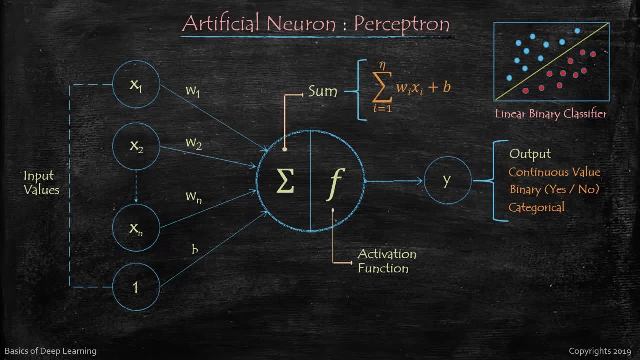 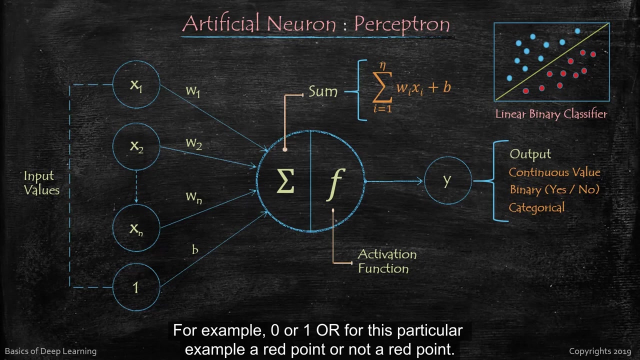 points, we are able to classify them into two categories. This is called as a linear separation, And the term binary is used as it classifies the data into two categories, for example, 0 or 1.. Or, for this particular example, a red point or 1.. 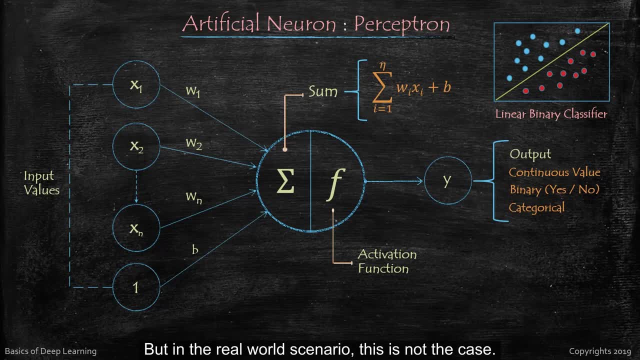 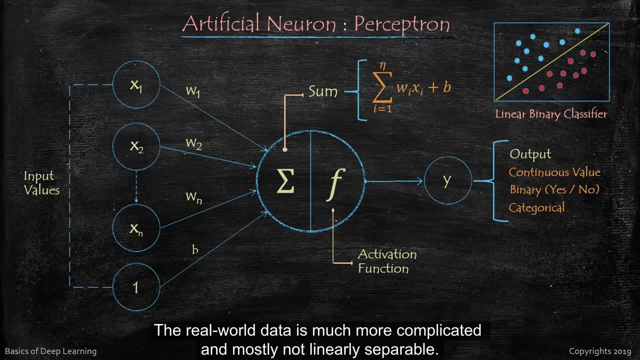 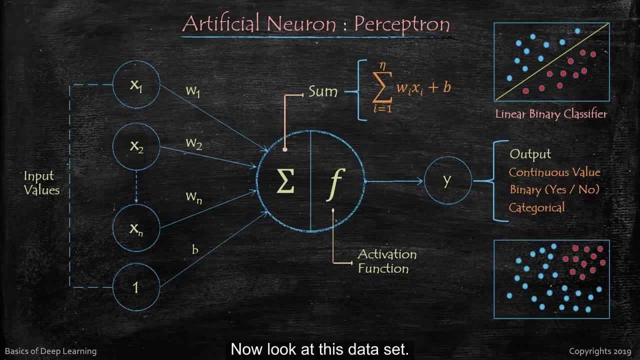 not a red point. But in real world scenario this is not the case. The real world data is much more complicated and mostly not linearly separable. Let's look at another example of data points. Now look at this data set. Here we cannot separate the data points linearly. or we can say: 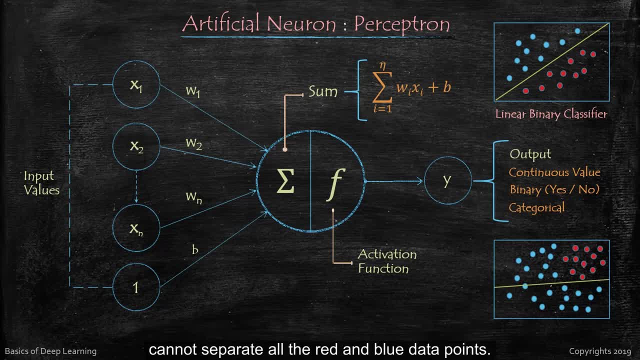 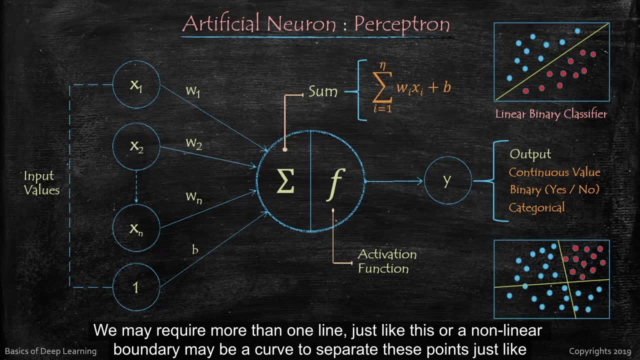 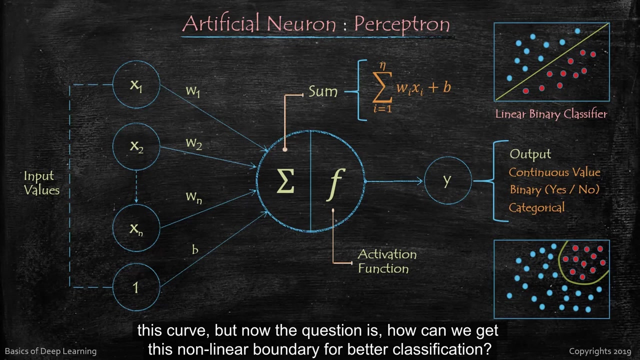 that a single line cannot separate all the red and blue data points. We may required more than one line, just like this, or a nonlinear boundary may be a curve to separate these points, just like this curve. But now the question is, how can we get this nonlinear boundary for better classification? 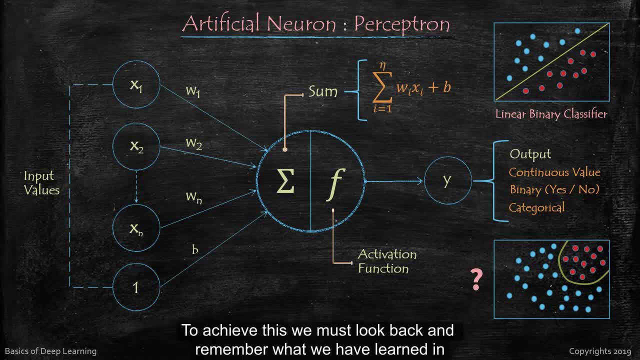 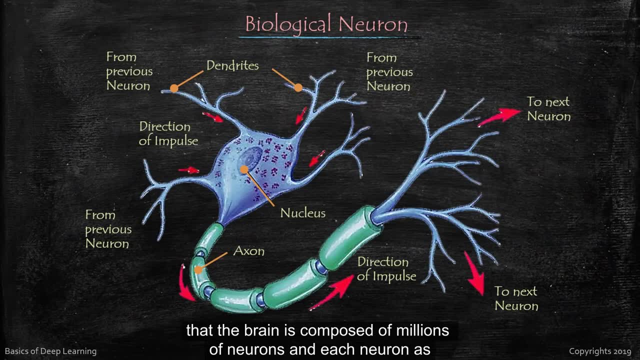 To achieve this, we must separate all the red points and blue data points. We must look back and remember what we have learned in our previous video. We have seen that the brain is composed of millions of neurons and each neuron, as connected to one another, receives a signal from. 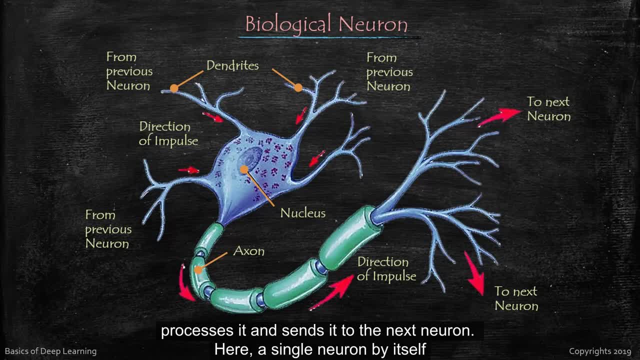 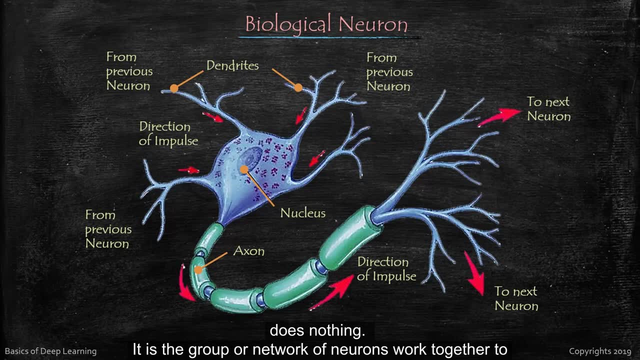 previous neurons, processes it and sends it to the next neuron. Here a single neuron by itself does nothing. It is the group or network of neurons work together to generate the desired output. If you take a real life example of a honey bee, you may have noticed that a bee by itself cannot do anything, But it is the 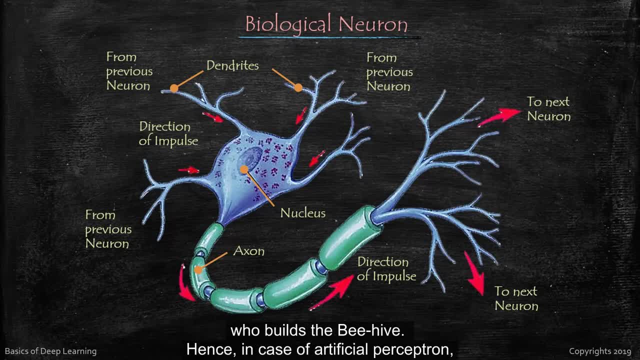 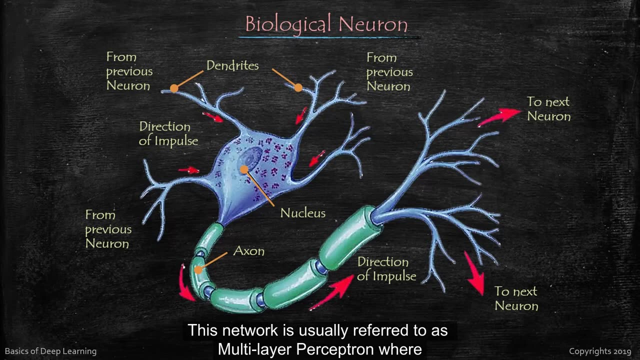 cluster of bees who builds the beehive. Hence, in case of artificial perceptron, we need to create a network of neurons to get the desired output. This network is traditionally referred to as multilayer perceptron, where each neuron is called node. 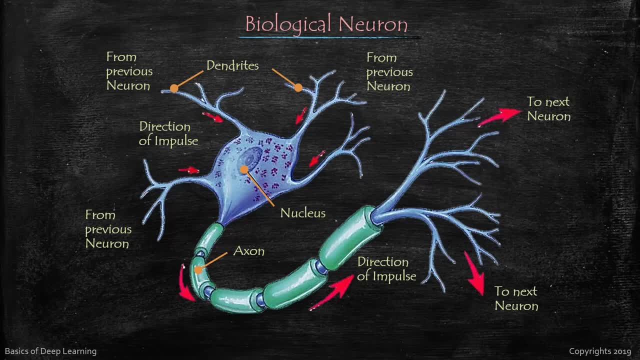 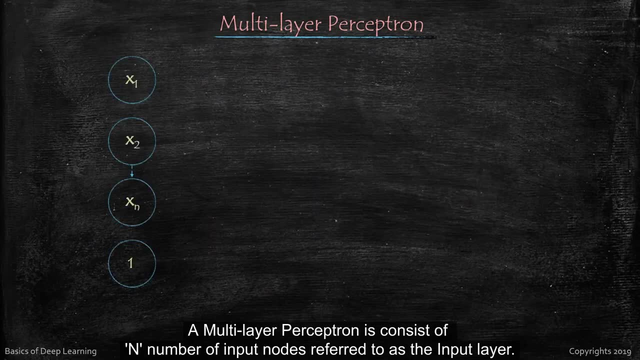 So let's have a look at a multilayer perceptron. A multi layer Perceptron is consists of n number of input nodes, referred to as the input layer, N number of nodes and N number of nodes it would refer to as the input layer are represented. 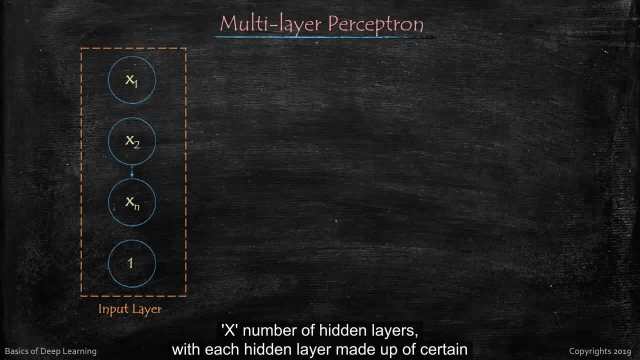 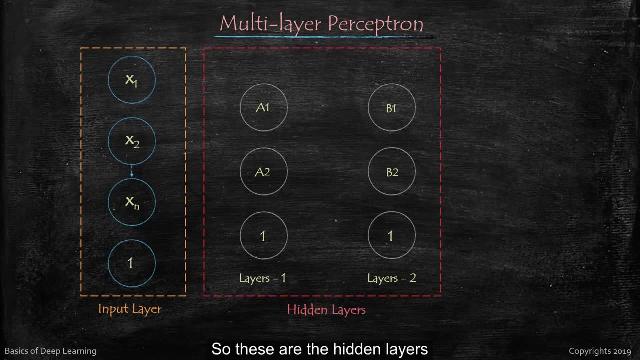 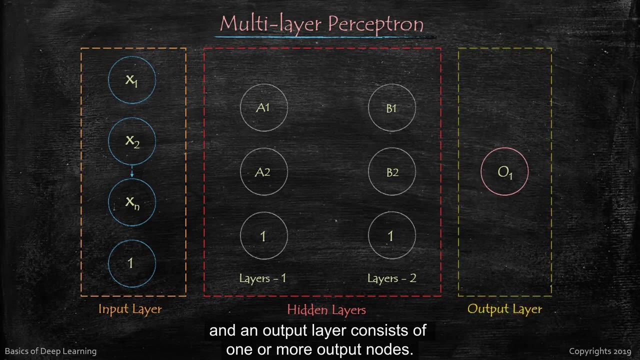 the row and the x number of hidden layers, with each hidden layer made up of certain number of processing nodes. So these are the hidden layers and an output layer consists of one or more output nodes. This network is fully connected network, where each node in the previous layer is connected to. 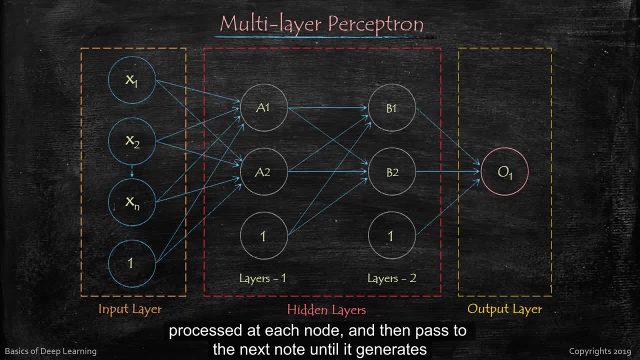 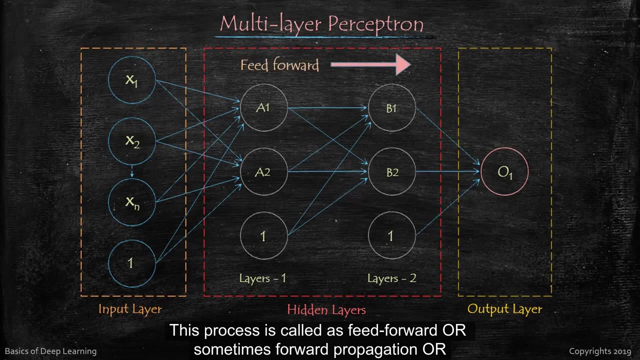 each node in the next layer. Inputs are processed at each node and then pass to the next node until it generates an output. This process is called as feed forward, or sometimes forward propagation or forward pass. You may hear these different names for the same process. 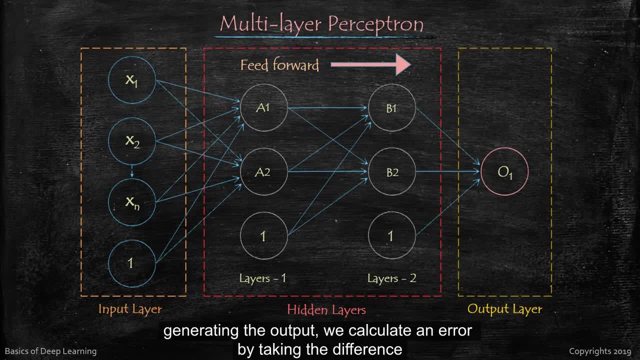 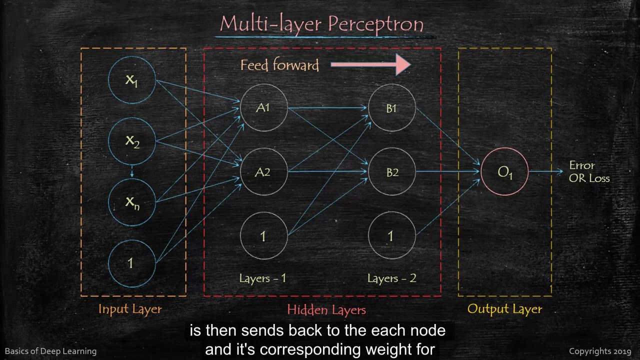 After generating the output, we calculate an error by taking the difference between output value and actual value. This error is then sends back to the each node and its corresponding weight for adjusting the weight value to reduce the error further. This process is called as back propagation using gradient descent, The feed forward and back. 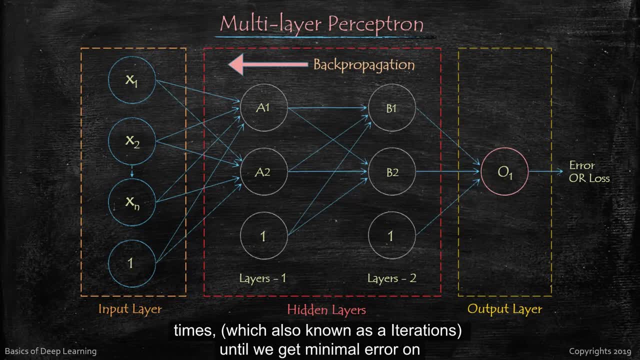 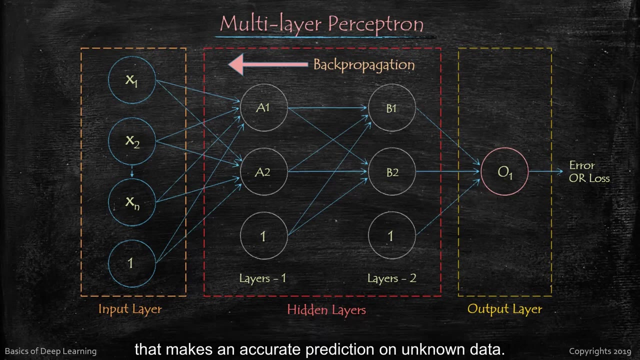 propagation is called as back propagation using gradient descent. The feed forward and back propagation process continues for several times, which also known as iterations, until we get minimal error on the output. This process is called training process and help us to create a model that makes an accurate prediction on unknown data. We will discuss forward pass. 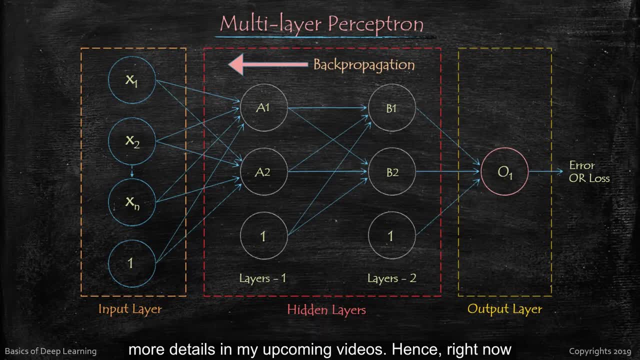 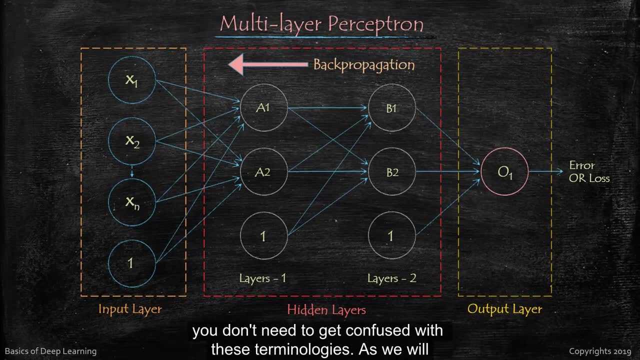 back propagation and gradient descent in more details in my upcoming videos. Hence, right now you don't need to get confused with these terminologies. As we will proceed ahead, you will slowly get acquainted with it. Now, before we will end this tutorial, 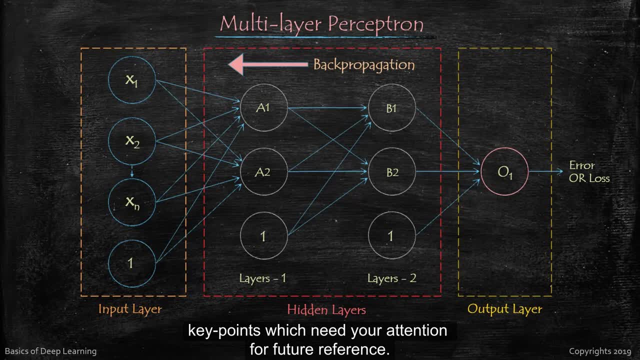 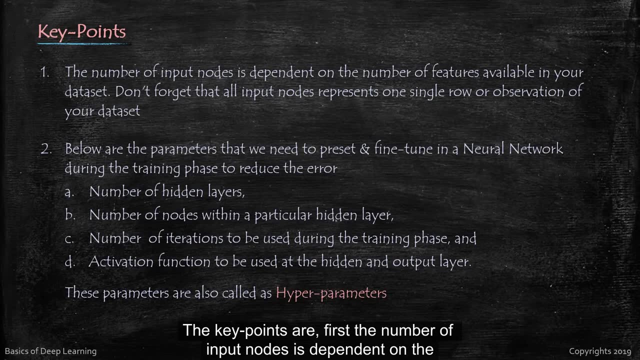 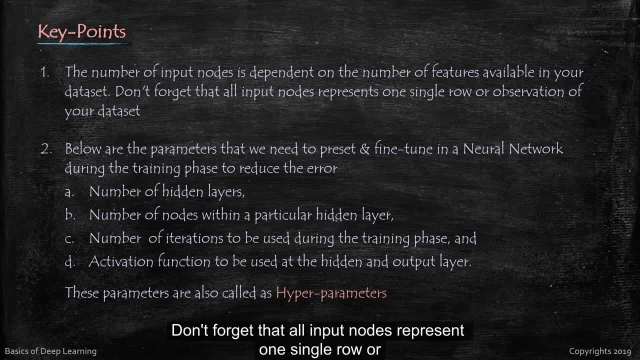 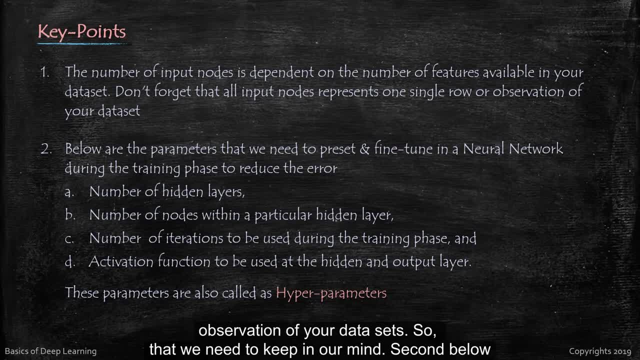 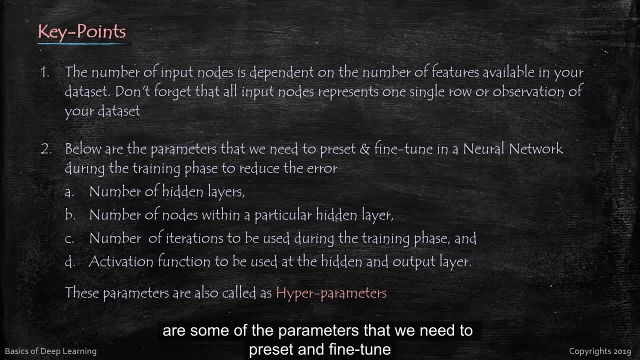 one single row or observation of your data sets So that we need to keep in our mind. Second, below are some of the parameters that we need to preset and fine-tune a neural network during the training phase to reduce the error. So first is number of hidden layers. 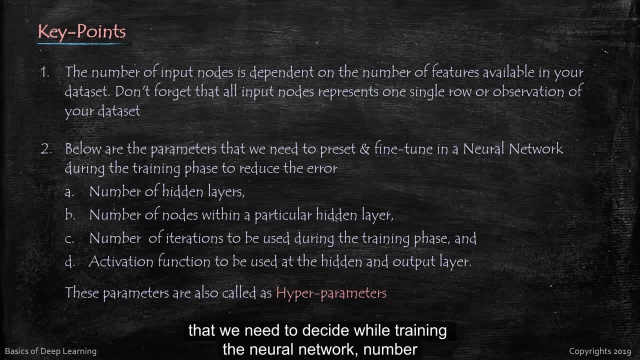 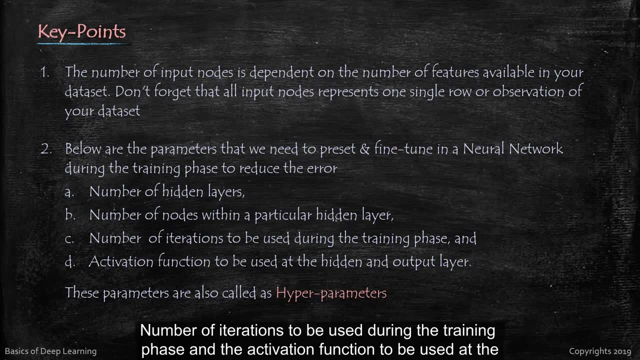 that we need to decide, while training the neural network, Number of nodes within a particular hidden layer, Number of iterations to be used during the training phase And the activation function to be used at the hidden and output layer. These parameters are also called as hyperparameters. 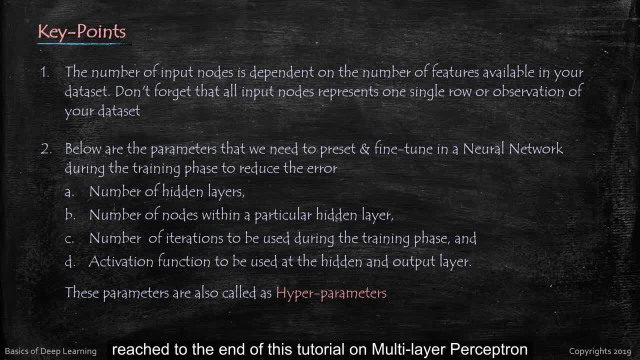 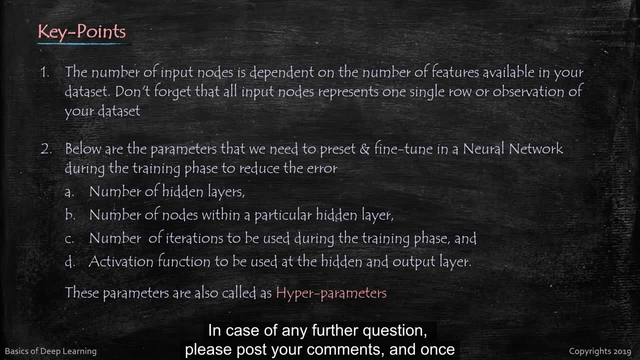 So this is it. We have reached to the end of this tutorial on multi-layer perceptron. In case of any further question, please post your comments And, once again, thank you for watching this video. Goodbye.